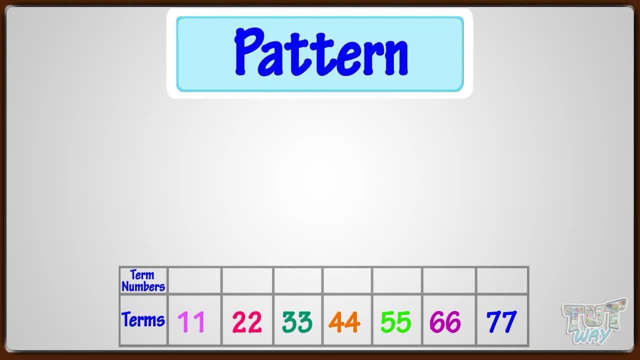 We have given term numbers from 1 to 7.. To each term, that is, there are 7 terms in this pattern, where term number of 11 is 1,, term number of 33 is 3, and so on. Now let's learn different types of patterns. 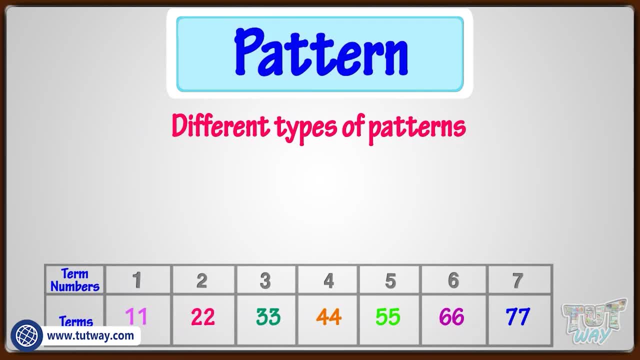 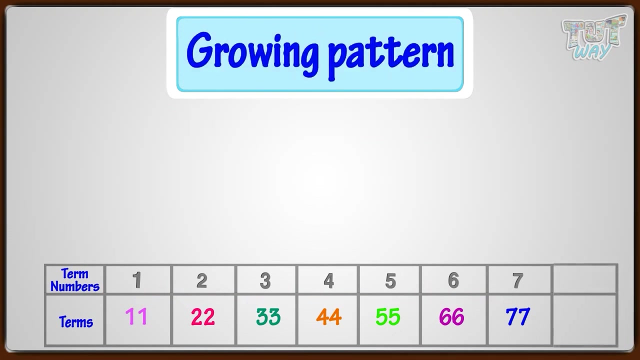 Kids. here is a pattern. Can you see and tell what type of pattern is it Here? the numbers are growing or increasing by each successive term. So it's a growing pattern. What should be the next, The next term in this growing pattern? 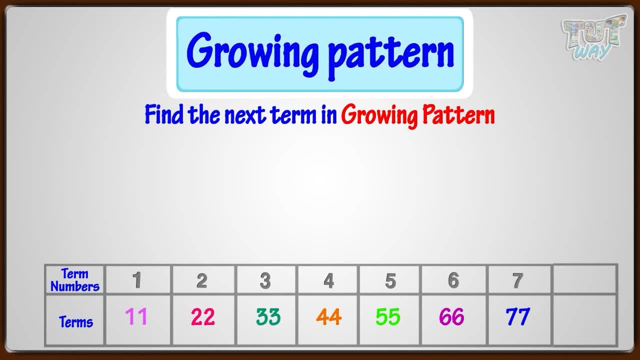 Here, with every successive term, we are adding 11 to the term. So to find out next term or the 8th term, we will add 11 to 77.. 77 plus 11, we get 88. So 8th term would be 88.. 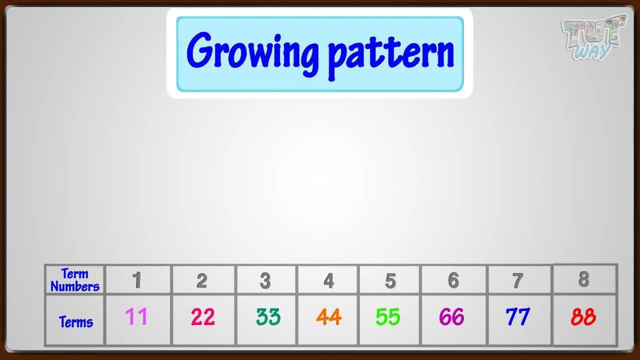 There is another way too. Here we can see that every term is term number multiplied by 11.. Like the term number 1 is 11 multiplied by 1, that is 11.. Term number 3 is 3 multiplied by 11, that is 33.. 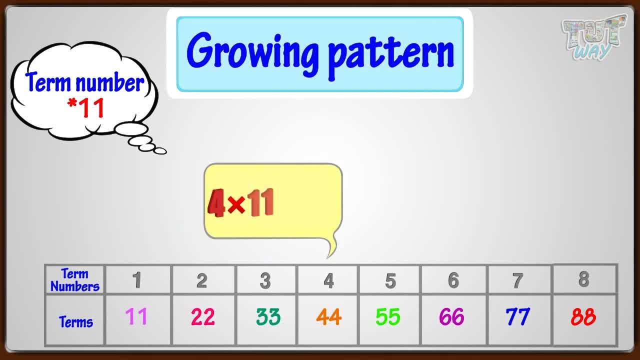 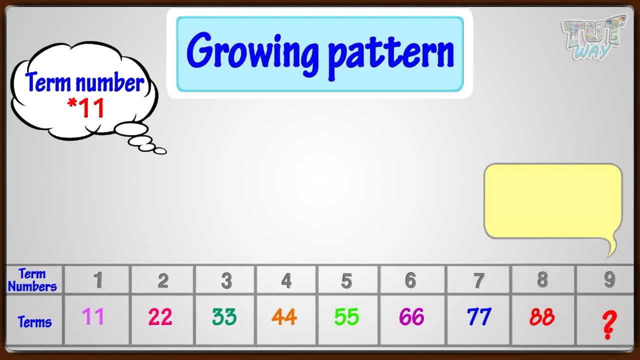 Term 4 is 4 multiplied by 3. multiplied by 11. That is 44. So if we have to find out the 9th term, we can say that it will be 9 multiplied by 11, which is equal to 99.. Now let's see more examples of growing patterns. 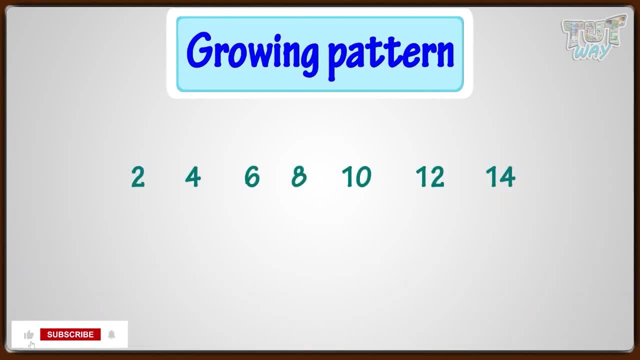 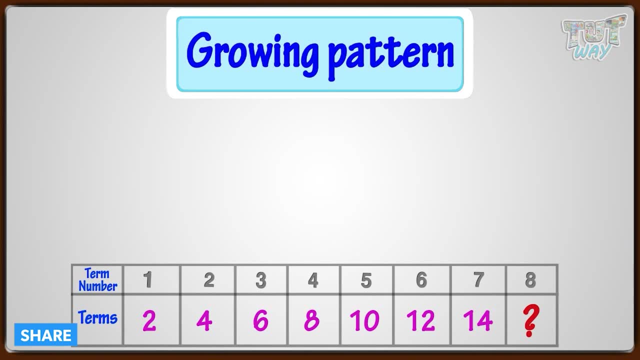 Here. what should be the next term Here? we have two ways to find the next term. One is we are adding 2 to every next term. 2 plus 2, we are getting 4.. 4 plus 2, we are getting 6.. 6 plus 2, we are getting 8.. Other way is: 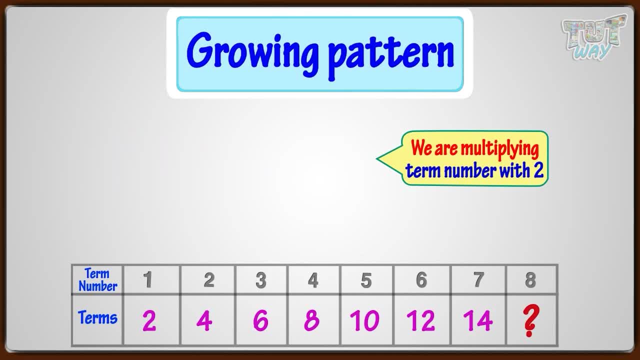 we are multiplying. We are multiplying term number with 2.. To get the term number 1, is 1 multiplied by 2.. Term number 2 is 2 multiplied by 2.. Term number 3 is 3 multiplied by 2.. Term number 4 is 4 multiplied by 2.. So find out the 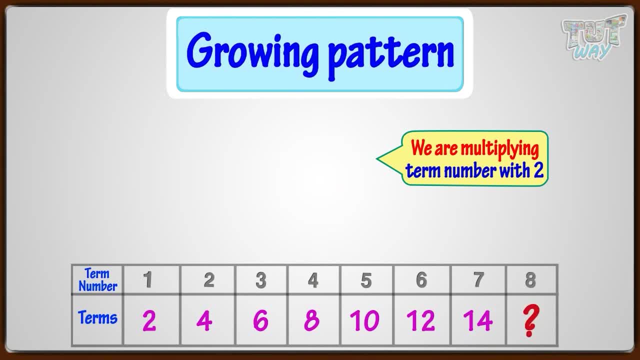 next term or 8th term. here We can multiply 8 with 2. We can get 16. or we can add 2 to the 7th term, That is, adding 2 to 14, we get 16.. Now have a look at more examples of growing patterns. 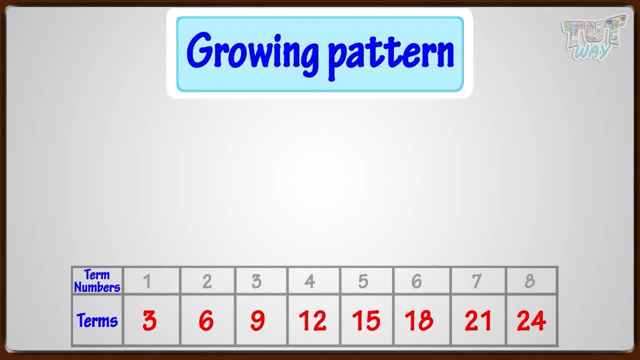 This is an example of growing patterns. Here we are adding 3 with each successive value. Now what should we do? We need to cleverly see how the above three patterns work. So let's Say we want to add 9,, 11,, 12,12 to any of the previous three terms that we had by ages 15 and 16. Now let's look at one more example of 7 patterns. This is an example of the other 7 patterns. Here we are adding 3 with each successive sixdee Six terms. This is an example of growing patterns. This setting contains number, addition and variation. 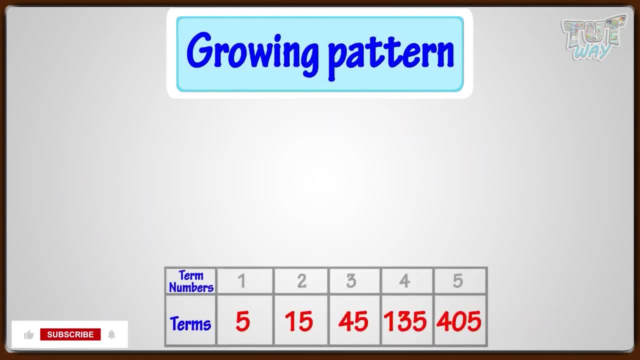 term. here is another growing pattern. here we are multiplying with three. like the first term is five, second term is first term multiplied with three. now the next term is 15 x 3 and the next term is 45 x 3 and the next term is 135 x 3 now. 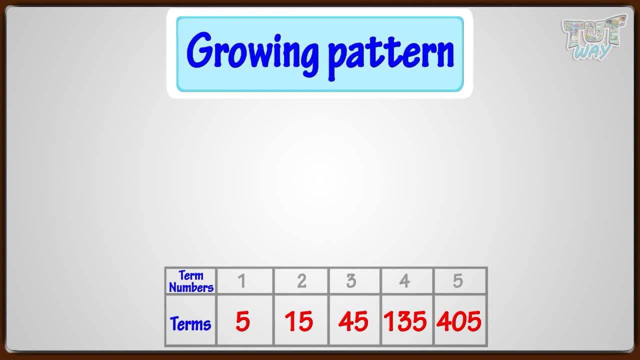 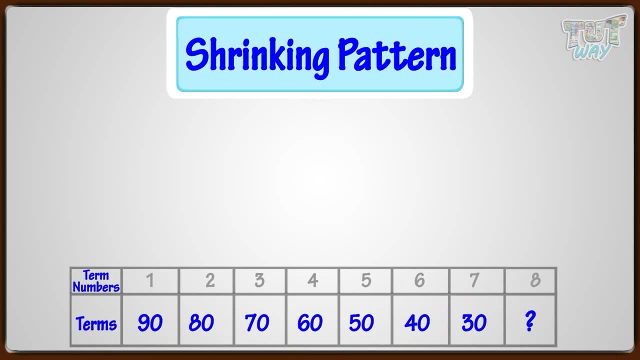 let's learn another type of pattern. it is shrinking pattern. here is an example. here are: And the numbers are decreasing with every term, exactly opposite to growing patterns, where the numbers increase by each successive term. Now let's find out what the next terms for this pattern is. 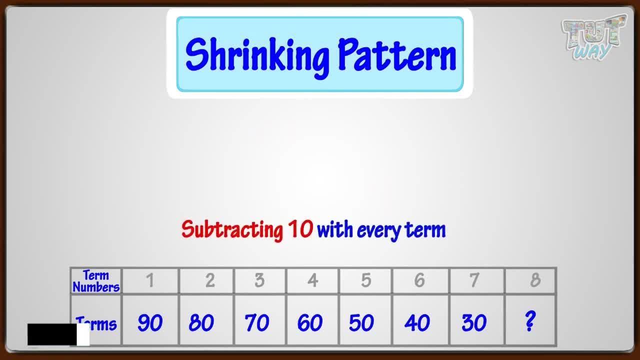 Here we are subtracting 10 with every term: 90 minus 10, we get 80.. 80 minus 10, we get 70.. 70 minus 10, we get 60. And so on. So next 8th term would be subtracting 10 from the 7th term. 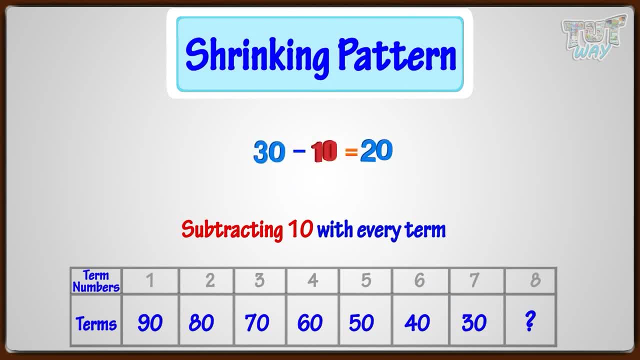 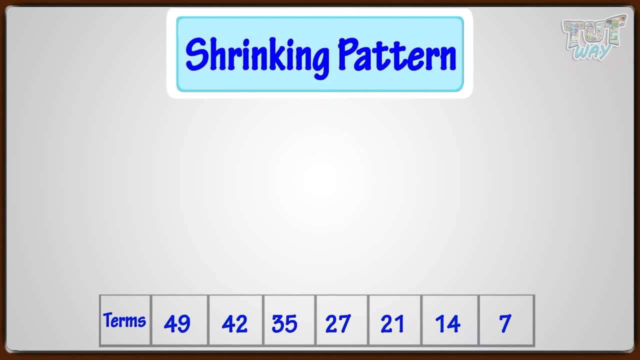 30 minus 10.. That is 20.. So 8th term would be 20.. Let's have a look at more shrinking patterns. Here we have a shrinking pattern Here. what should be the next term? See, here we are subtracting 7 with every successive term. 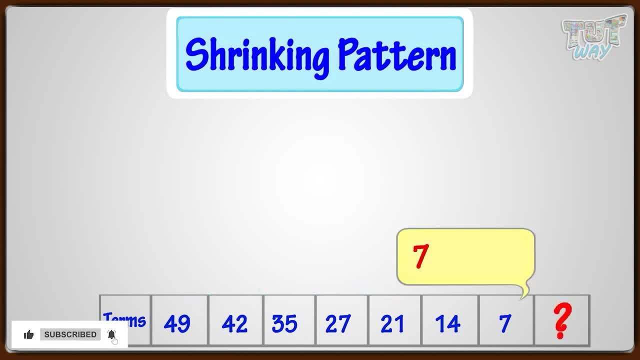 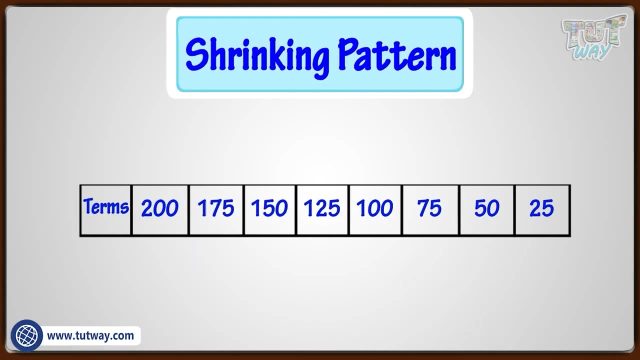 So the next term would be 7 minus 7, that is, The next term would be 0.. Here we have another shrinking pattern. Each term decreases with the growing term number. So these are shrinking patterns. Let's have a look at some other type of patterns. 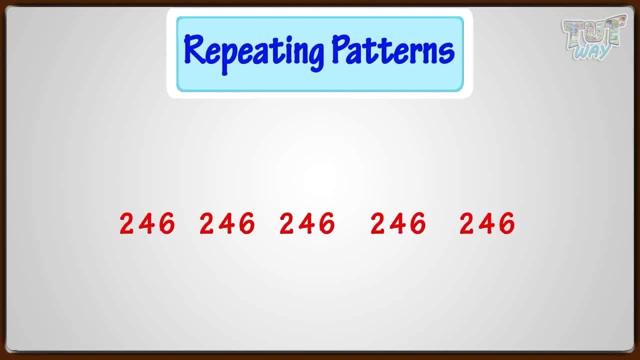 They are repeating patterns Here, the number 2,, 4, 6 and getting repeated, So it's a repeating pattern as the number 2, 4, 6 are repeating What should come in the blank space here. In any repeating pattern we first find the core pattern. 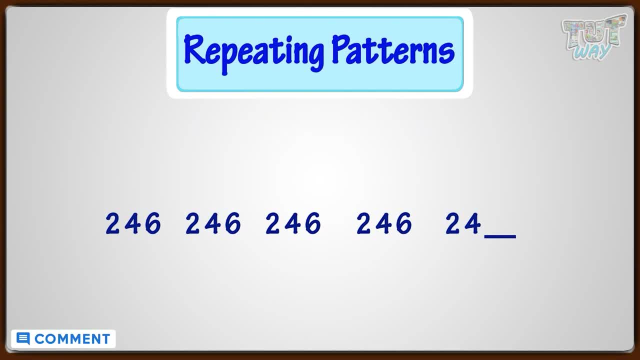 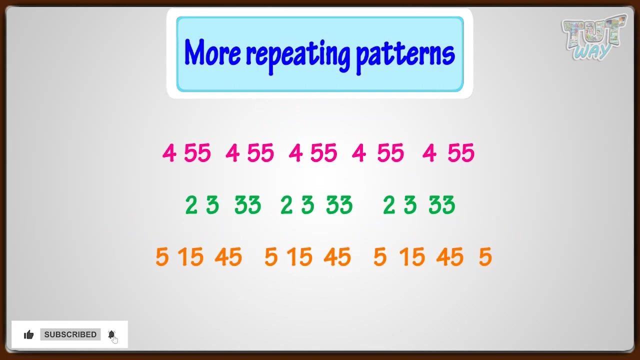 That is the term that's getting repeated, And then we can repeat it any times to grow the pattern. Here the core pattern is 2, 4, 6.. So according to core pattern, 6 would come after 4.. Now let's have a look at more repeating patterns. 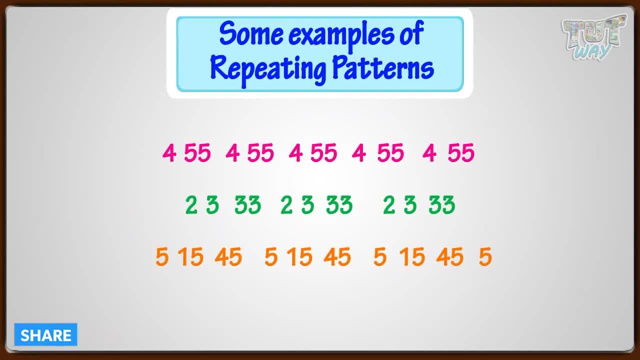 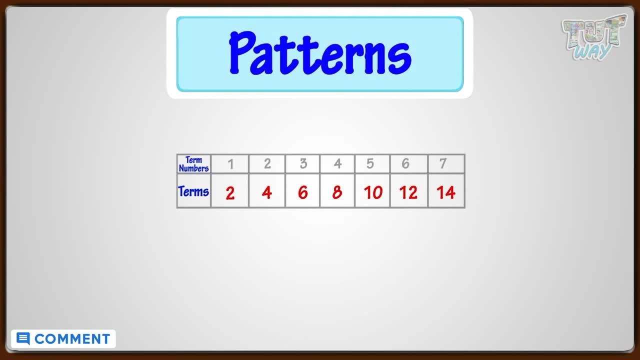 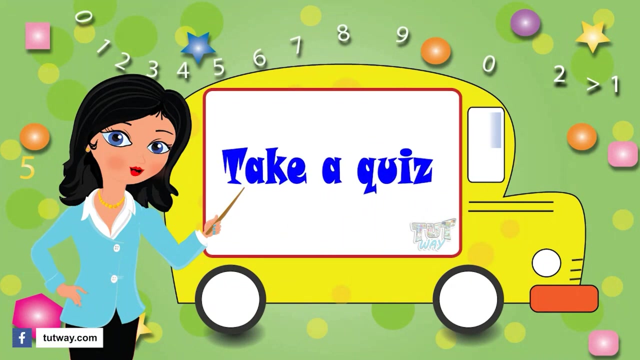 These are some examples of repeating patterns. So, kids, today we learned about patterns, Terms, term numbers and 3 types of patterns: growing patterns, shrinking patterns, repeating patterns. Now go ahead and take a quiz to learn more. Bye, bye, Thank you so much for watching.